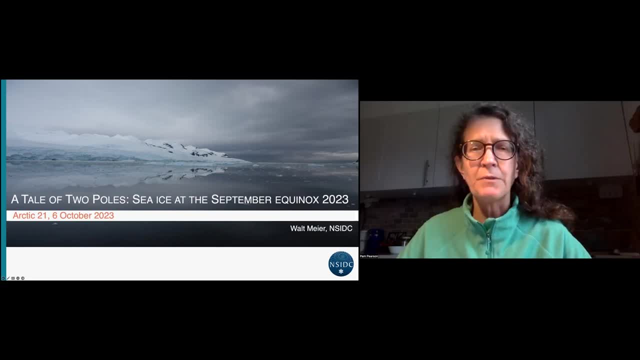 So certainly something is going on also in Antarctica and, almost in recognition of this, to give a bit of a preview of the state of the cryosphere report, this year that used to be called that chapter, Arctic sea ice. This year it's going to be called simply sea ice, because we're going to be covering Antarctica almost as much as we do the Arctic. 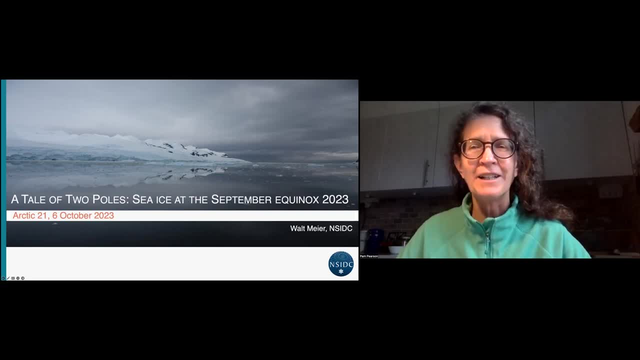 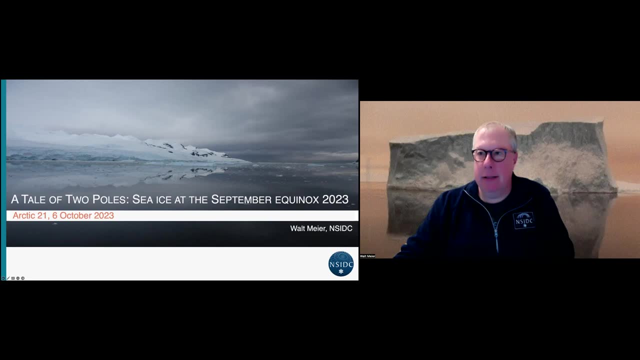 So, with that said, Walt has a wonderful title and I'll let you take it away, All right. All right, everyone hear me and see the slides. Perfect, Okay, great, And yeah, I haven't really had a chance to. I kind of threw these together so I'm not totally sure how long it is. 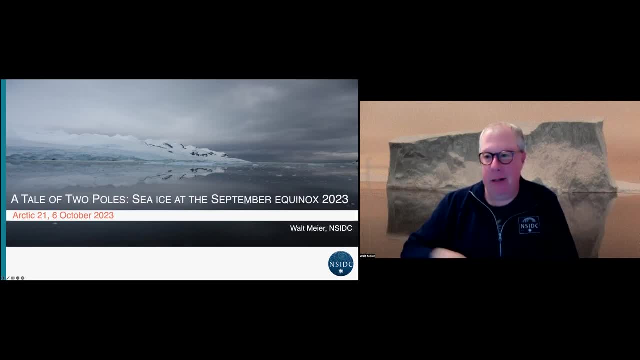 So if I'm running on a bit long, feel free to interrupt and tell me to speed it up or finish up, But hopefully this will take away about 20 minutes. so 15, 20 minutes. So, as Pam mentioned, you know it's been an interesting. 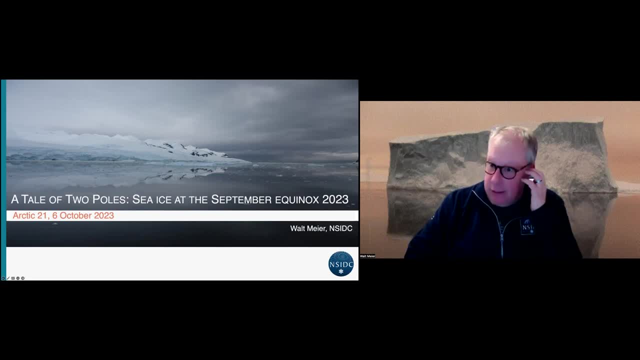 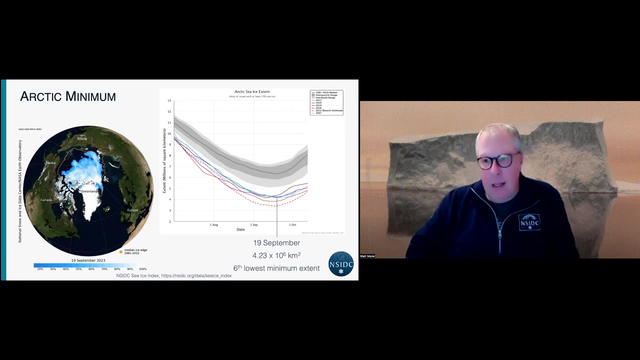 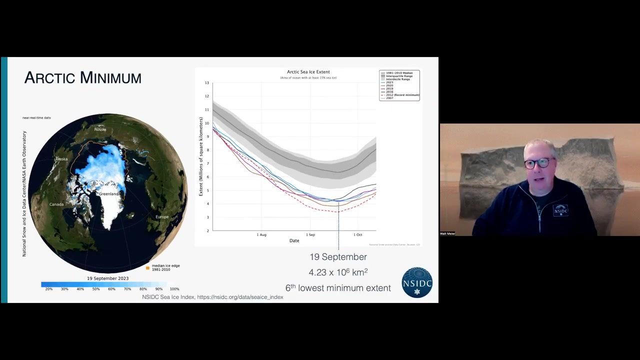 September, you know, equinox period, particularly in the Antarctic. but I will start, Oh yeah, Oh, there we go. Oops, Start in the Arctic, as we usually do, And it was, you know it's starting to. I feel like it's almost like a kind of a boring Arctic, especially, I guess, in light of the Antarctic. 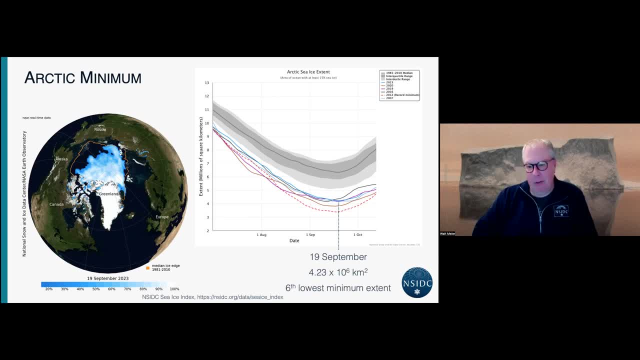 It was, you know, another very low minimum. It was the sixth lowest minimum extent on September 19th, which is fairly late, about a week later than normal, And 4.23 million square kilometers. So you know it was certainly low, but it wasn't particularly near a record low. 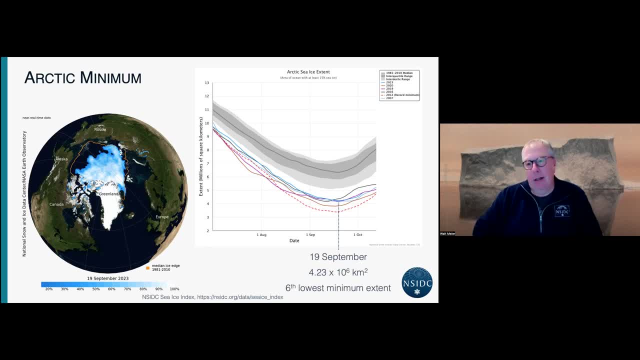 You can see the 2012 in the red dash on the right daily plot there, But you know it was in the ballpark of Several others and all quite low. this year, like many years. you know the Western Arctic really opened up the Beaufort, the Chukchi, the East Siberian Sea- far lower than average extent. you know vast areas of open water. 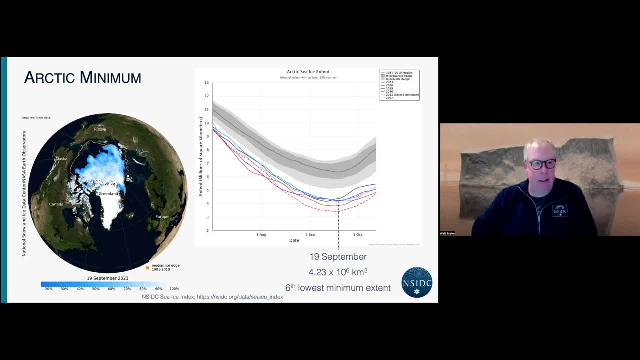 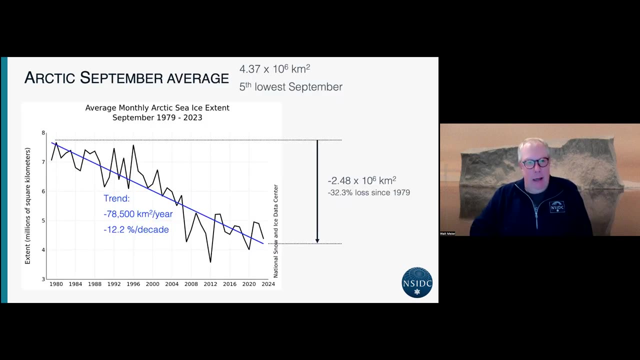 That's, you know, kind of in line with what we've seen many years. in recent years, You know the pattern is slightly different, but There's oftentimes been a lot of open water in that area. Looking at the average extent for this is September. 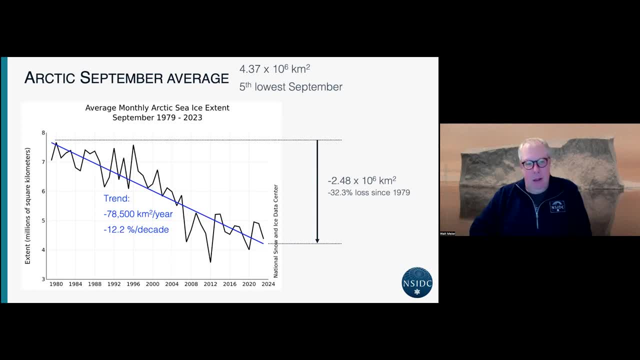 This is the average September extent. now, You see, you know a very clear, strong downward trend. It hasn't changed too much in recent years. It's on the order of, you know, 75 to 80,000 square kilometers per year, about 12 percent per decade. 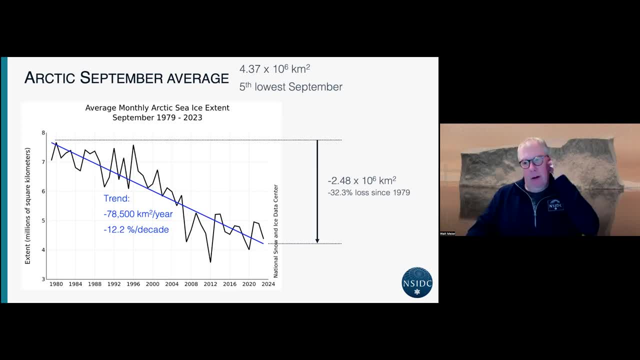 Overall, if you look at the trend line, we're down. We've lost about 200.. Half a million square kilometers, which is about a third of the extent of the at the at the September monthly extent. So again, you know this year was was down from the last couple of years, just slightly above the trend line. 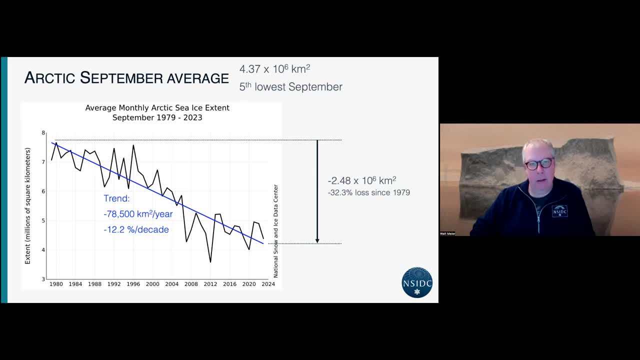 But yet another. you know another low year. But something that we've been noticing for for a while now is That, Well, we've got this long term Trend is very clear, very strong since about 2007.. We've seen a lot of variability. 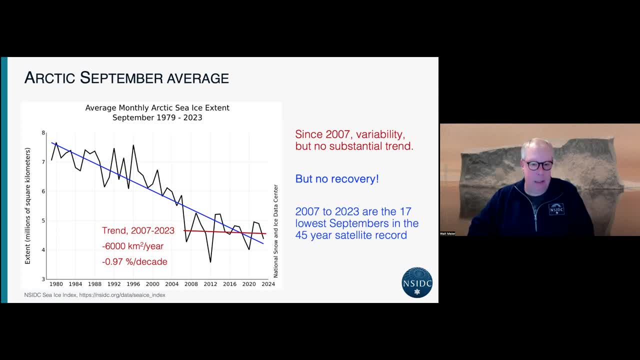 We've seen a record low, 2012.. We've seen a couple others that were quite close. Twenty twenty was the second lowest. Twenty sixteen was nearly as low as as as 2007.. This year was quite low And but if we look at that- that trend from 2007 to 2023, it's basically flat. 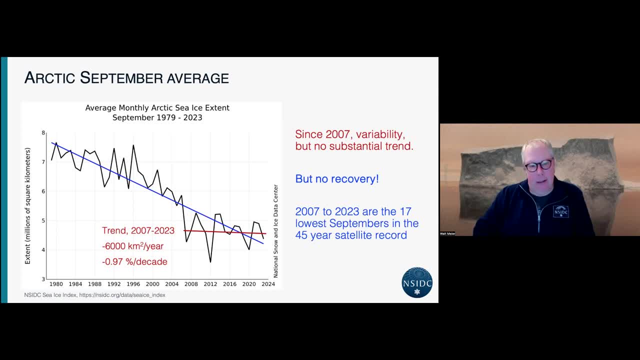 It's just Barely negative. It's not statistically significant: less than one percent per decade. So we're in this kind of pause, in some sense of the downward trend, where it hasn't continued downward. But I want to emphasize that there's no recovery. 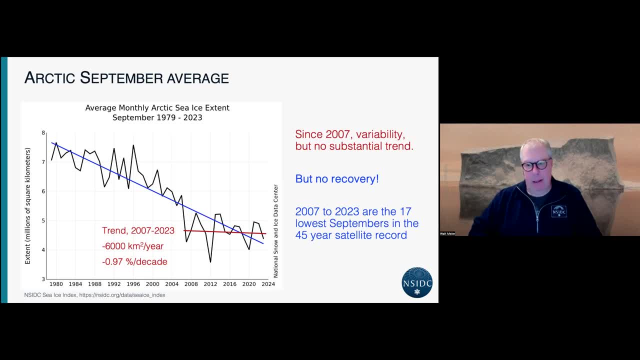 It's up and down a bit, but it's. it's flat, There's. it's not heading back up towards 1990s or 1980s level And, in fact, the last 17 years, which is 2007.. 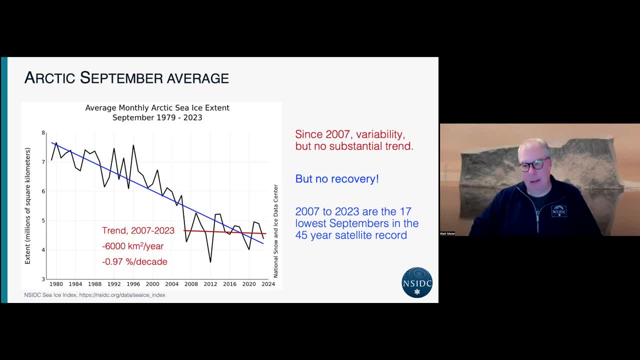 To 2023 are the 17 lowest Septembers in the 40 year, 45 year satellite record. That's not something you would see by chance. That's clearly indicating that there's a fundamentally changed Arctic sea ice environment. But we're there, at least for the moment, in a bit of a pause in terms of a downward, downward trend. 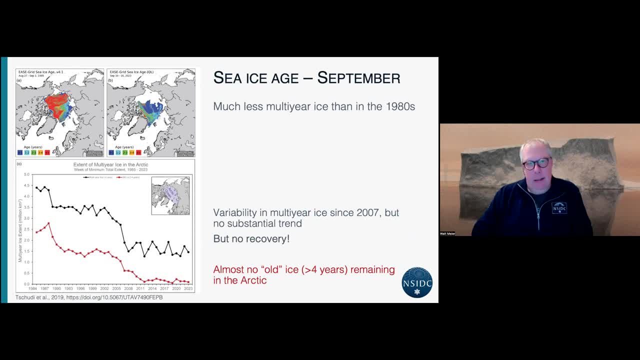 Another thing in part of the reason for that, I think, Is this- is the fact that we've we've lost a lot of the what I would say we've lost a lot of the easy ice. the ice that's lower latitudes, more near the coast, gets more solar energy during the summertime. 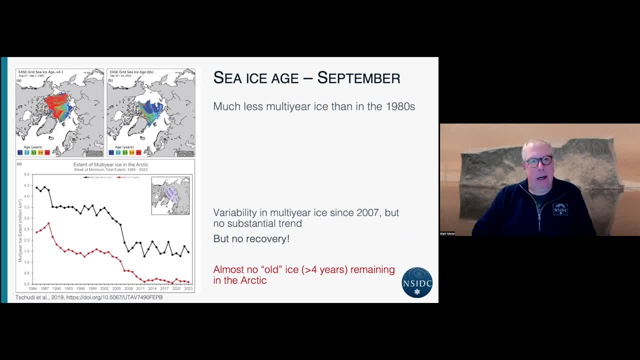 It's more first year ice, more seasonal ice and thinner ice. It's also ice in the, at least in the Siberian side, where it tends to be getting infected across the Arctic and out, so that ice tends to be thinner. And so while we've seen, very clearly, you know, a dramatic change in the in the age of the ice cover and the upper left, making a five dominated over much of the Arctic, is the four greater than four years old, four plus years old ice. 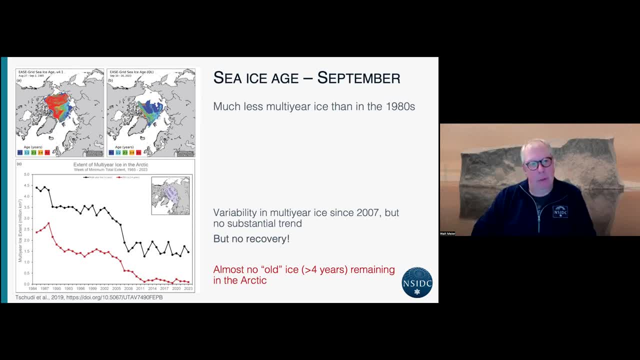 And that's almost non-existent now. There's just really not much left. Looking at the extent year by year, This is At the minimum the multi-year ice and the and then the old ice, the greater than four years. If you look at the multi-year ice it looks kind of like the the sea ice extent. 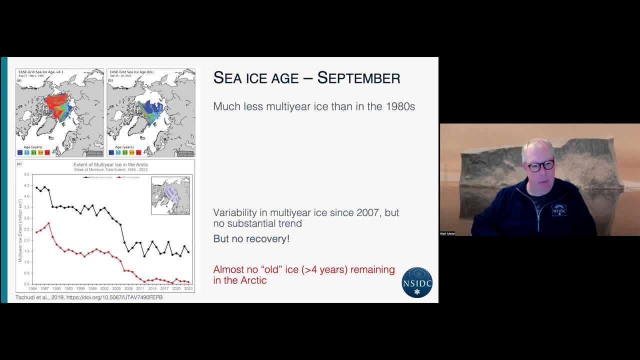 There's a lot of up and down. There isn't really much of a trend. I didn't, I didn't put a trend on there, but basically since 2007, it's it's essentially zero, But again, there's no recovery. 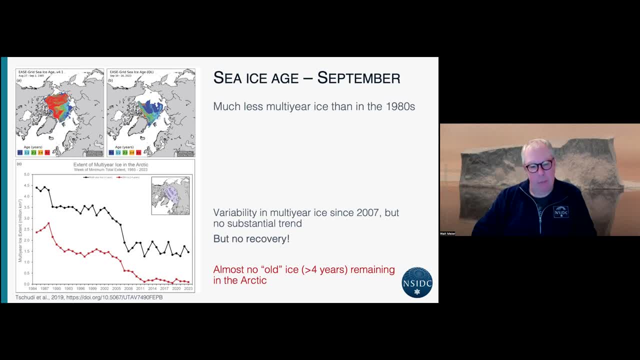 It just bounces up and down every two or three years And it's kind of been flat. The, The old ice which I said you know again, is virtually disappeared, especially since about 2012 when we had that record low minimum extent. 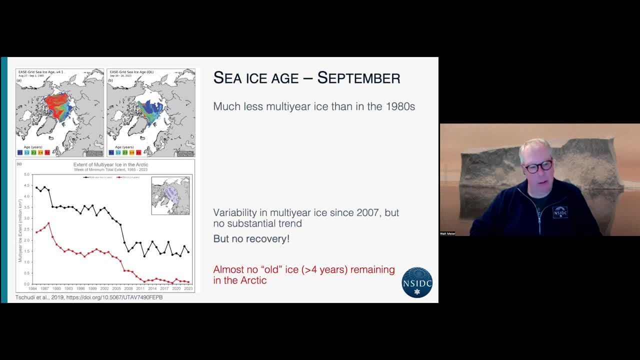 And it's just, you know, hovering really kind of just above zero. about 100,000 to 200,000 square kilometers compared to upwards of two million square kilometers is what it used to be. So there just isn't any old ice left. 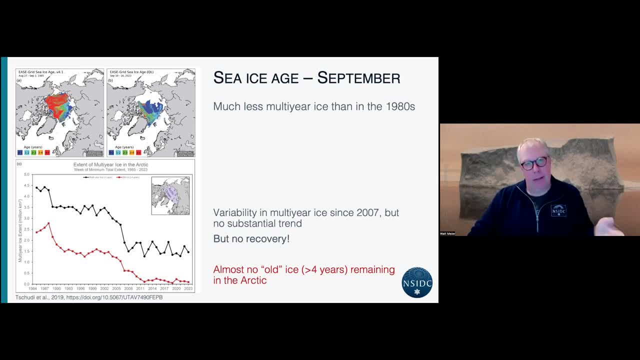 So there's the multi-year, you know ice. that survived a summer and it might survive Another summer or two, But that's it. It's not really staying around in the Arctic, unlike it used to. It's it's the lifetime of Arctic sea ice is is really much less than it used to be. 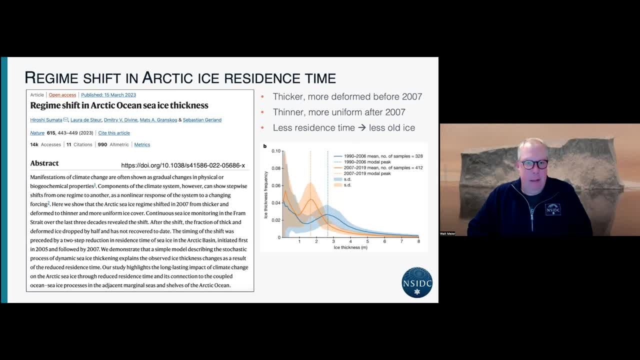 And you know the cause of this is. you know, I think you've got a thinner ice cover. Obviously it's warmer temperatures. There was this interesting paper- Folks haven't seen it- Hiroshi Samada And others that looked at this kind of a regime shift starting in 2007, where basically the the ice thickness distribution has changed. 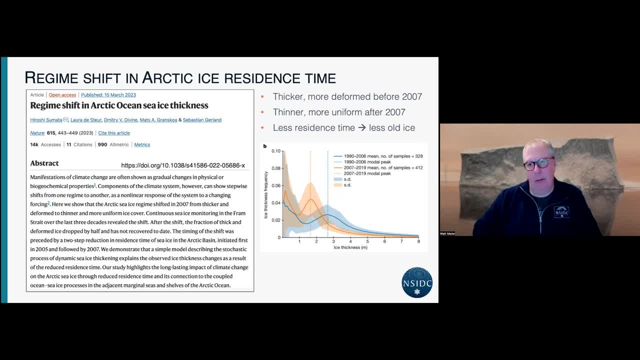 We went from a thicker, more deformed ice cover into a thinner, more uniform ice cover And the ice is staying around less, less time There's. the ice motion is faster and it's moving across the Arctic and out of the Arctic faster. 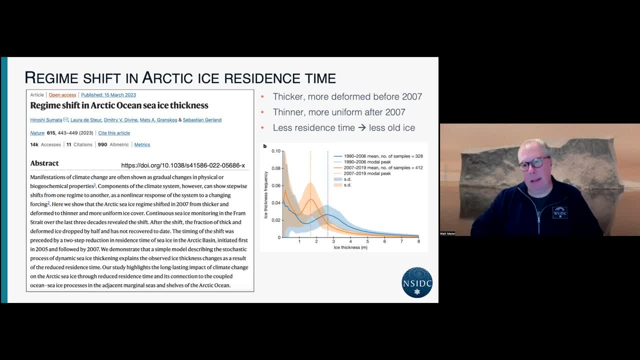 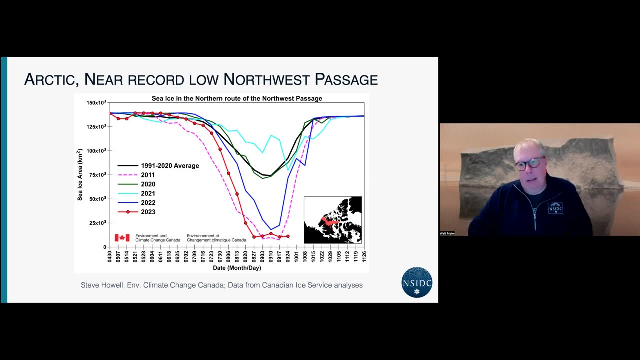 And so it's just not staying around long enough to build up Thickness like it used to. So the lower residence time is is kind of an aspect of this regime shift that we've seen. I just before I move on to the Antarctic, another interesting thing that always is of interest, or interest of many people: the Northwest Passage. you know that's not as important as the Northern Sea Route, Siberian side, in terms of shipping. 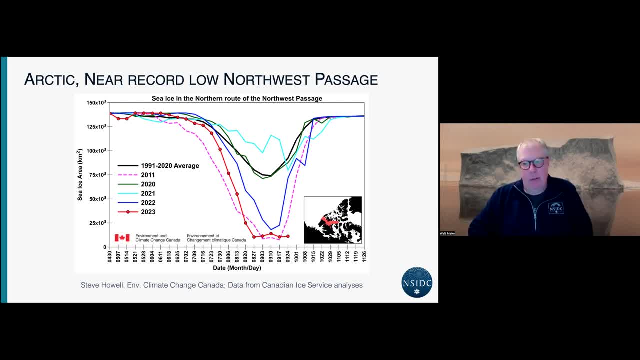 But you know it has, it has. It has a fabled history to it and this year was a particularly low year in the Northwest Passage. This is this little red area. This is like the northern route of the Northwest Passage through. this is Baffin Bay. 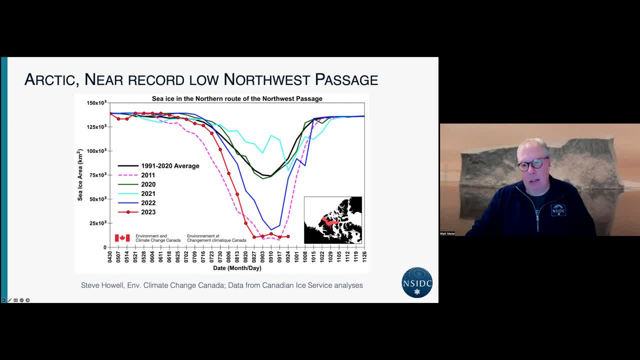 You can see my mouse over on the right and then the Bulkard Sea, And this red shaded area is where the extent is, or the area is being calculated. And 2011 was the record almost completely cleared out. This year It basically did the same thing, but it didn't quite reach 2011 levels, so it's the second lowest in the records. 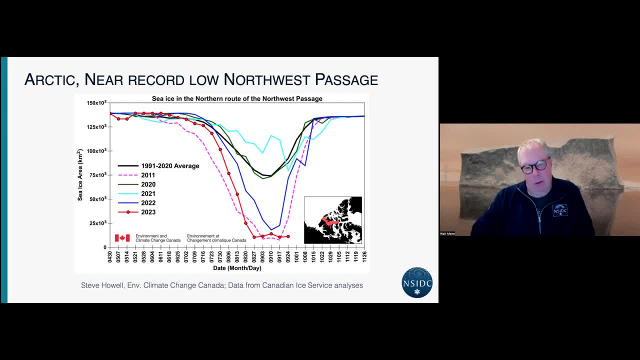 And these are from the Canadian Ice Service ice charts. Steve Howell at Environment Canada put these together for us, And it's nice to see that the Northwest Passage is a little bit tricky to consider in terms of a climate indicator, because it's not only dependent on the, you know, the kind of the melt within the passage, but also the inflow of ice. 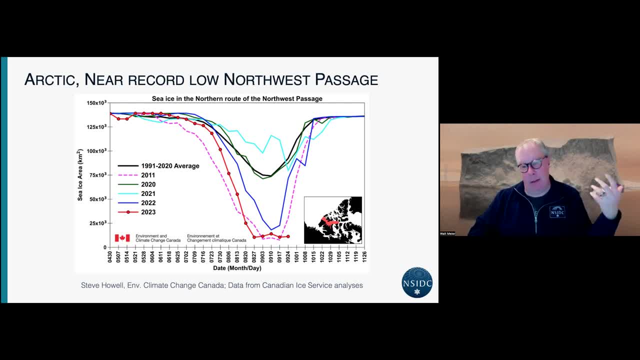 from the north. that can kind of fill up the passage, even if it's a warm year. so the northwest passage extent doesn't necessarily correlate with the overall um. arctic total arctic sea ice extent um, but this was a pretty extreme year in terms of that. it was pretty open all the way through, except that. 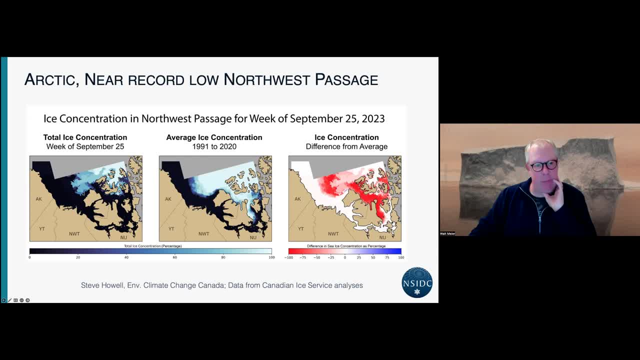 interestingly, there the passage itself was open, but the mouth of the passage on the western side, the mcclure strait, um, there was basically ice that kind of hung around throughout the winter. um it it, you know, even along the coast of banks island. so you really actually couldn't quite get. 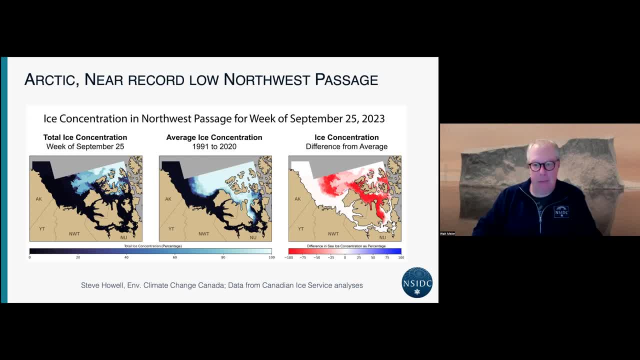 through without having some ice, getting being able to get through the ice- maybe not an icebreaker necessarily, um, and it did sort of go away from the coast a little bit for a little while. um, you might have been able to sneak along the coast of banks island over here. 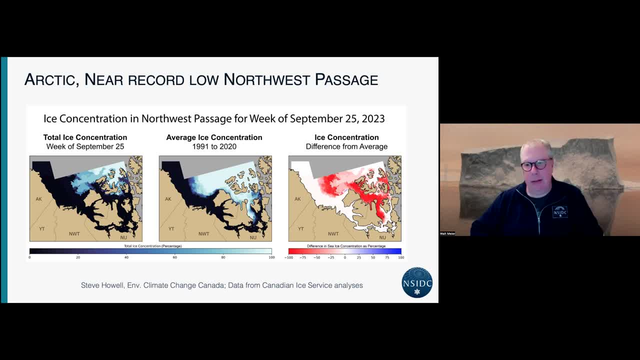 um, but you know, so it's kind of an interesting. you know, the passage itself was was open, um, but you would hit the end and it would be a roadblock there, basically, but the southern route which goes through narrower, shallower channels all the way, all the way down south, along the coast, that was. 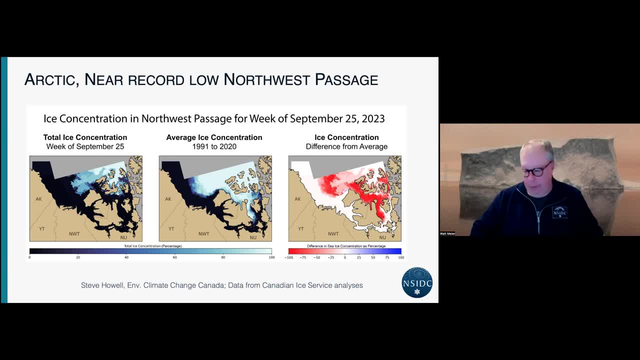 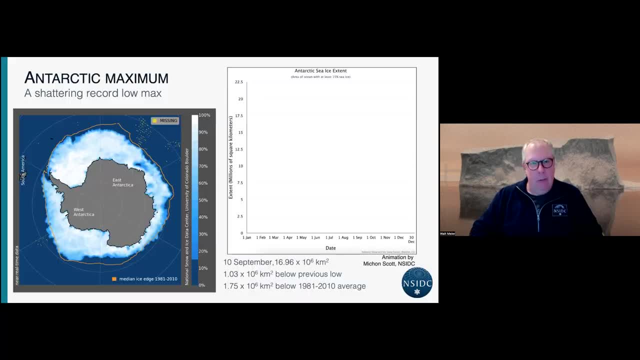 wide open, um for several weeks and i think still is wide open. so, um, now turning towards the, the south, um, you know, where things are a little more interesting? um, as folks are probably aware, um, so, uh, this is the extent on the. uh, i forgot to put the date on. 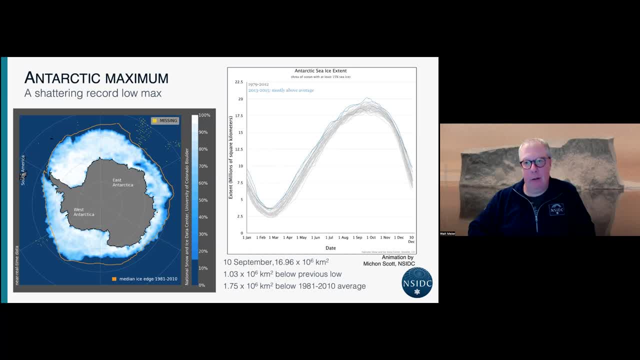 there, but that's september 10th, which is when the minimum was, or maximum was. if you look at this animation- hopefully this is showing up for folks- um, we, you know, we went from being pretty high in like the 2013 to 2015 era. over those three years, we actually had record high maximums. um, and then 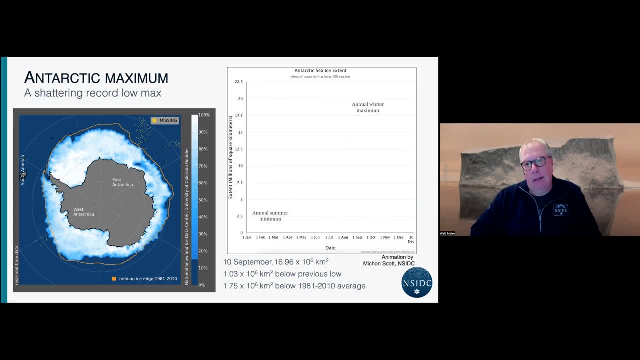 it was this kind of regime shift where we suddenly dropped um, but soon after the maximum in 2016, and it's been mostly lower than average and even record low um since then. um 2017 was a record low minimum, uh, 2022 was a record low minimum and then this year was another record low minimum. 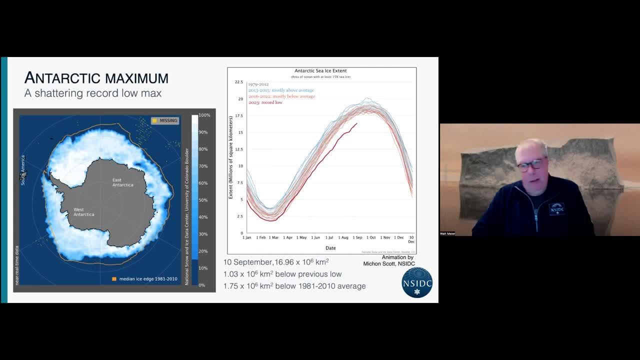 back in, you know, like late february. what really grabs one's attention, as you've probably seen, is the. the growth season through the autumn and winter in the in the antarctic was just really slow. uh, it just lagged behind. you can see how the- the 2023 line here just starts sticking out. 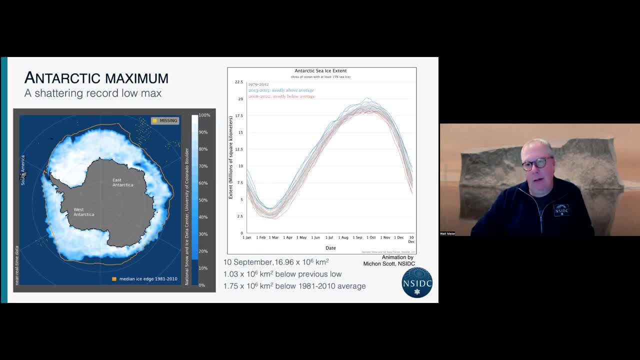 like a sore thumb. um, compared to all the other years, it's just way outside the normal variability that we've seen in the satellite record, which goes back to 1979. so there's over a million year square kilometers below the previous low. so it's just a smashing record low, um, it's, you know, it's. 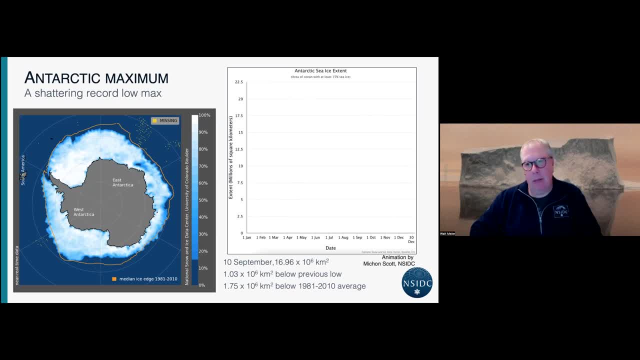 on the order of what 2007 did in the arctic for the minimum um in in 2012. um, but we haven't seen this type of record in that scale, um in the antarctic at all. um, you know, almost one and three quarters million square kilometers below the, the, the average extent. so um, just uh, i think. 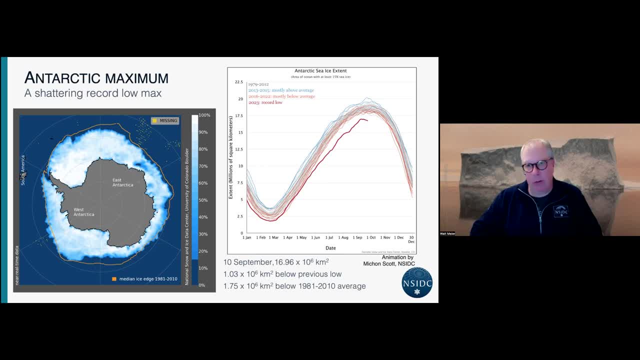 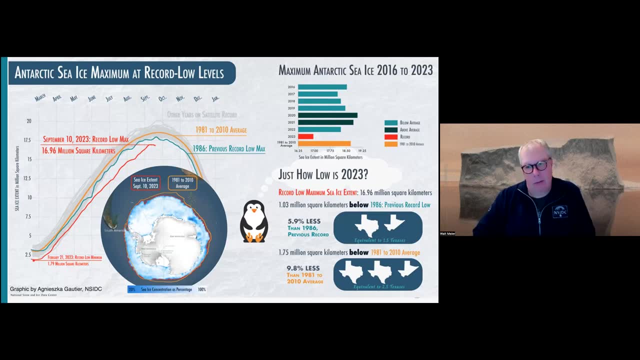 uh, low maximum and slow growth. um, this is just another um way of uh looking at it. this is a nice graphic that uh one of our communications team member, agneska gotia, put together, um, just to illustrate it. you know it's- the percentages are somewhat small because there's so much ice, you're. 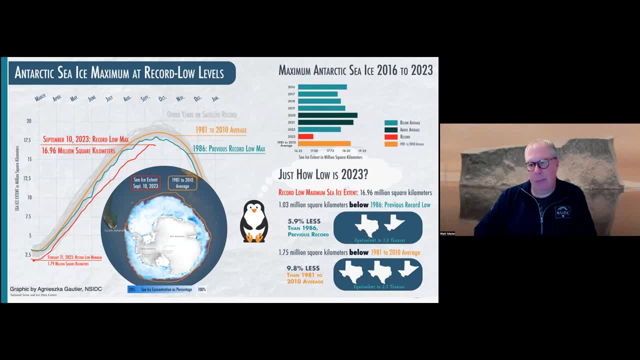 when you're talking 18 million square kilometers and you're down a couple million square kilometers. it's not all that much in percentage but it's a huge number. um, you know about one and a half. texas is below the previous record in about two and a half. 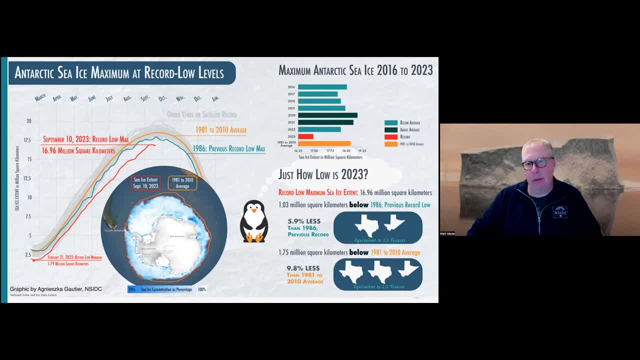 texas is below the average. um, you can see some of the recent ones. uh, recent years up in the upper right, you know 2020 and 2021 were, you know, a little bit above average. nothing extreme, but other than that, um, we've been quite, quite a bit below average in terms of our maximums, as well as. 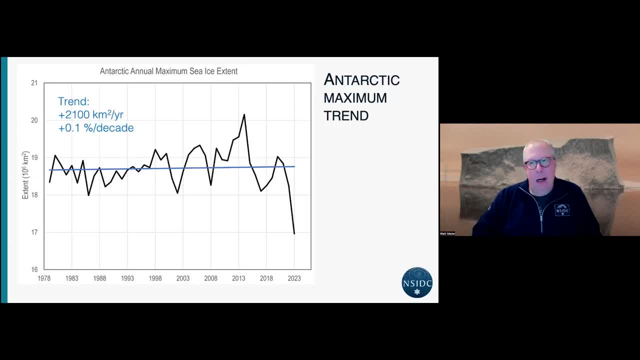 the rest of the year really, um, we look at the trend, you know, just looking at the maximum, you know, again, this year really sticks out how, how it totally falls out of line of anything that we've seen. um, you know, the 2014, that peak with the maximum was that was our highest maximum. that was pretty extreme, um, but we're as much as. 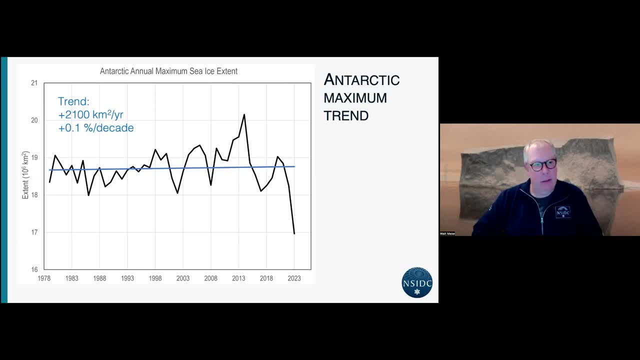 that or more than than that, over below the average um in terms of the minimum, the trend interesting, still positive, just barely. it's, it's not specifically significant. i, i don't know, i don't. i would essentially call it a zero trend um. it's a. you know, when you calculate the statistics, the 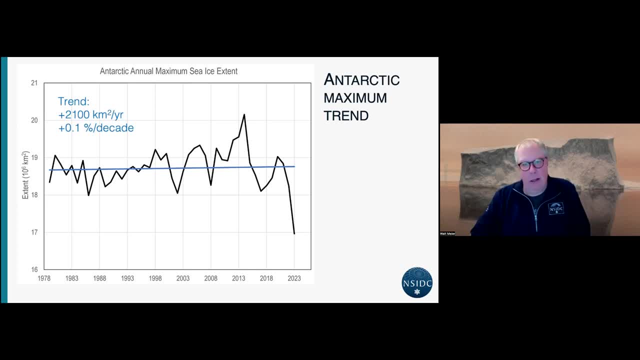 number comes out 2 000 square 2 100 square kilometers per year um, but that's not statistically significant, but it's. it's down quite a bit from like. in 2014, um, it was still a small trend, um was more on the order of about one to one and a half percent per decade um, but now it's- it's gone, it's. 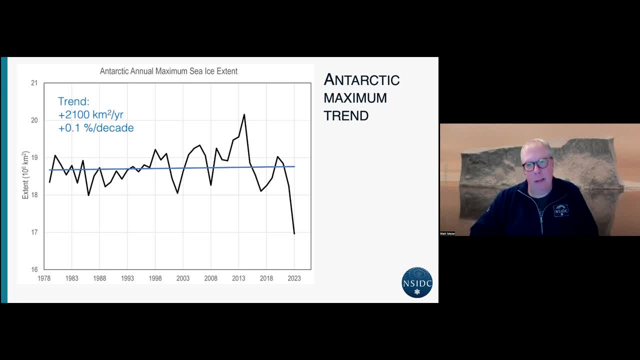 dropped back to almost zero. so we're trending towards a negative trend, um, at least in the last uh, few years, um, but overall, since 1979, we're not there um so, but you know, one of the questions is this: is there's a lot of variability in the antarctic, our satellite? 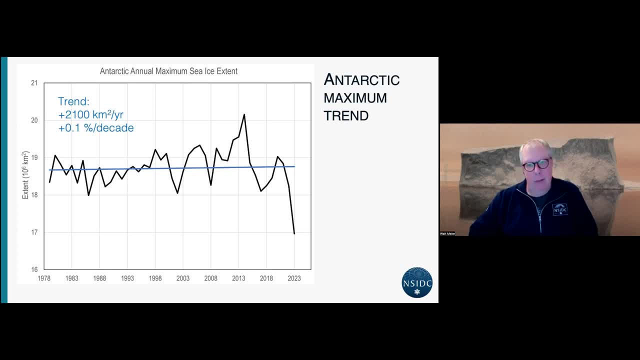 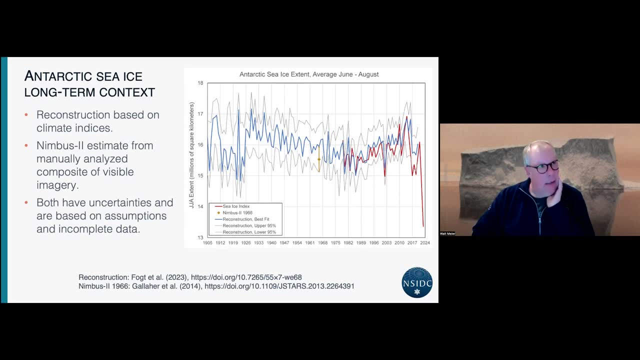 records 45 years. that's a pretty long record, um, but is that long enough to really capture the variability um in the antarctic sea ice? and yeah, i got a lot of questions um from folks um about a paper that i i was a co-author on, uh, dave gallagher. 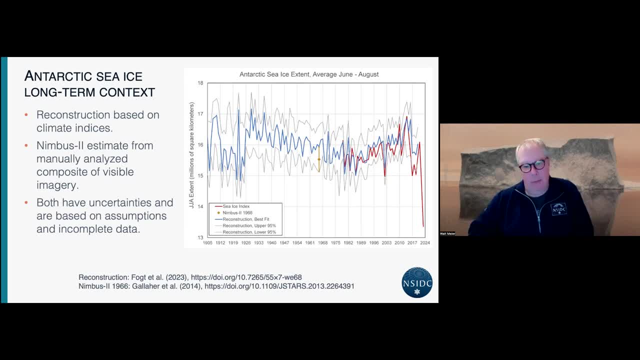 and dave and garrett campbell. dave galler was the lead author back in 19 in 2014, looking at early nimbus 2 satellite data, um from 1966. we were able to recover that data, digitize it and then we attempted to try to get a an ice extent out of it. um. i didn't put the example. 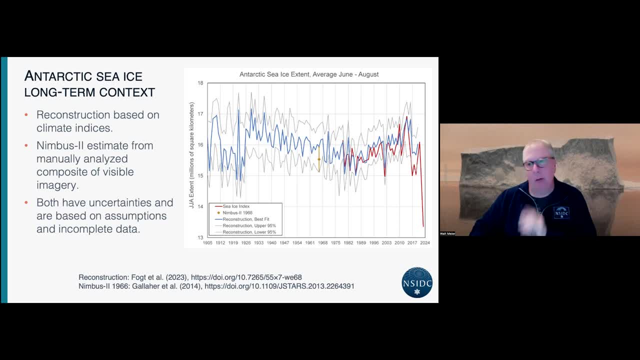 of the image. it's on our our most recent news website, uh, news post, um, but it it. you know, when we calculated the extent for august, it was pretty low. um, it was on par with what we saw in august this year, um, so there was several people that were kind. 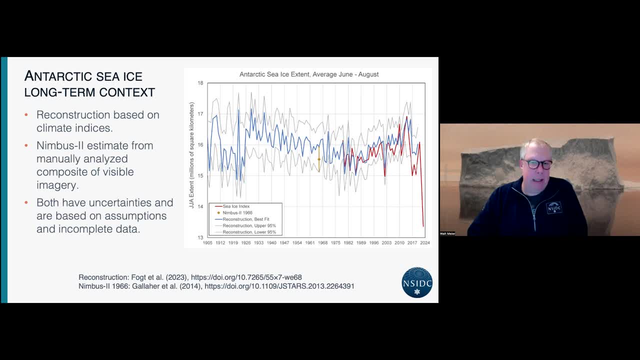 of you know, like i said, getting in touch, going like: well, hey, you're saying this is really shocking, but in 1966 it looks like you have a number that's somewhat similar. well, if you actually look at the numbers, um, you know, our august is actually still lower in 2020 and we're still 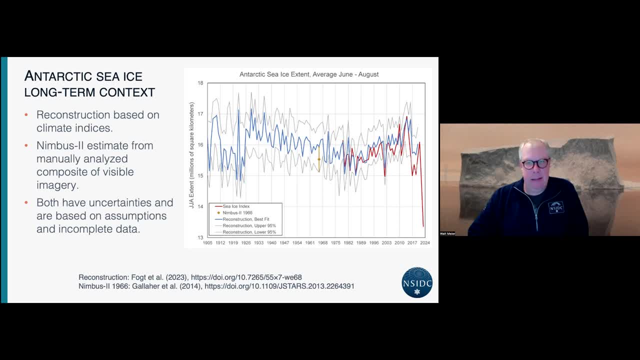 looking at the numbers in 2023. they were kind of a lot of people were comparing the 66 data to the september maximum um, and we didn't have data. there were no data in september from nimbus 2 in 1966. so you know, so that it wasn't completely apples to apples comparison. for one thing, 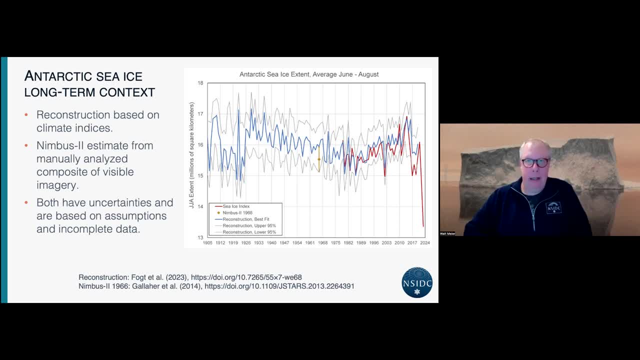 the other thing is it's it's visible imagery, it's it's old data. you know we did a lot of work to digitize it, to try to improve the quality and try to get something out of it, but it's still the quality is is good. 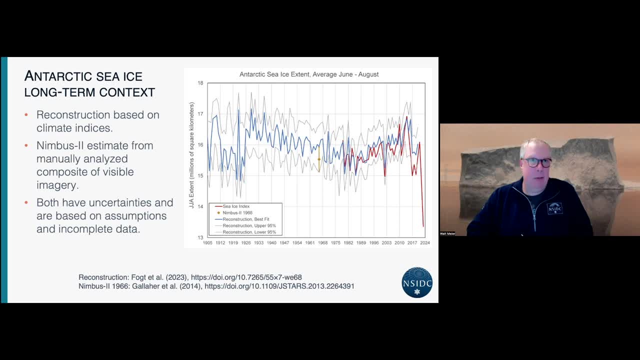 it's kind of iffy and it's, it's scattered. the images are scattered. you can't get data under clouds, so, um, it's, it's i. i hesitate to put too much emphasis on it, and one of the things that really is a telltale sign of the- at least the august data- is that the august value, that that. 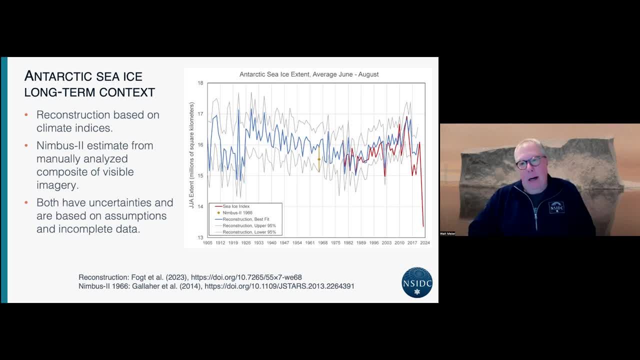 was derived from that nimbus 2? um in 1966 was actually lower than than the july data, um than the july extent estimate, and that just doesn't make sense. um, as you're going through the winter, um, you, just you're not going to, you're, you're really not. 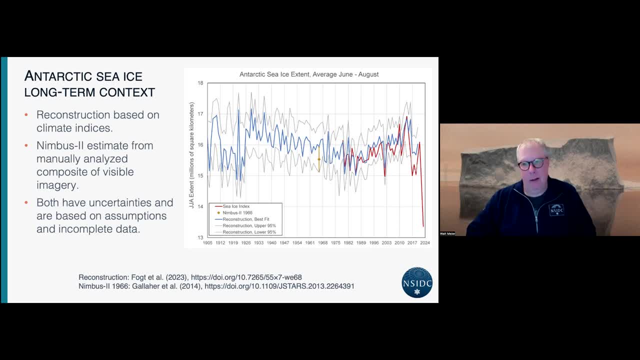 going to have, you're not going to lose ice from one month to the other. um, it just doesn't make sense. so the august value is pretty suspect. um, and the june and july values are more in line with, like kind of the historical norms. um, so it probably was just some bad data in august. 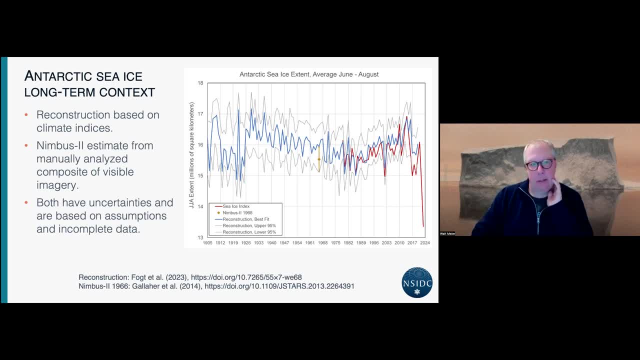 but i also um wanted to look at the longer term context in light of another new data set from ryan folk at ohio state and others, um that we just published- it, as i can see, a couple months ago. it's a, it's a reconstruction, so they basically took 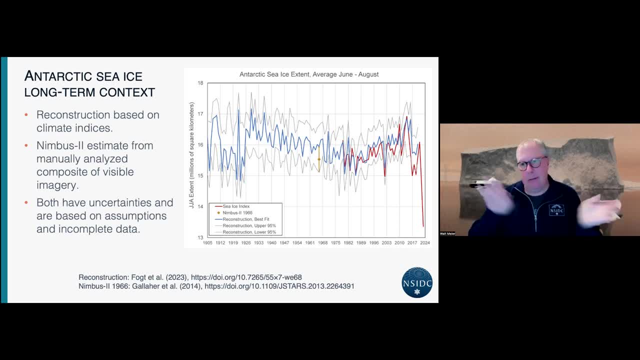 various. you know climate indices and reanalysis and and you know things, records that go back to 1905, um, and then you related those to the observed sea ice and then use that as a proxy to drive sea ice extent on a seasonal basis. so june, july and august, the 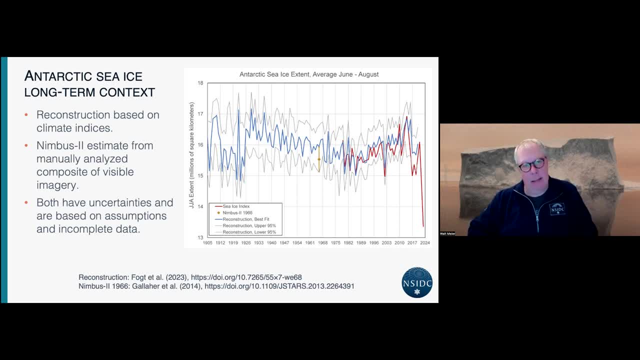 three-month average um in all other three-month seasons um. so i plotted that against um, our satellite record, which is in red, the reconstructions in blue, they they're best fit. and then they also calculated an upper and lower 95 percentile bound um. so you can kind of see: 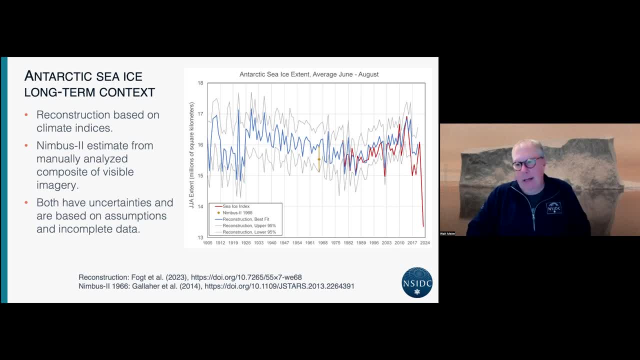 those and again our current um extent in 2023. you know, for june, july and august, just you know, dropping off a cliff compared to anything seen in um in since 1905 in the reconstruction and then also plotted. there is the nimbus data for 1966 in the gold diamond with the uncertainty range and i just took like 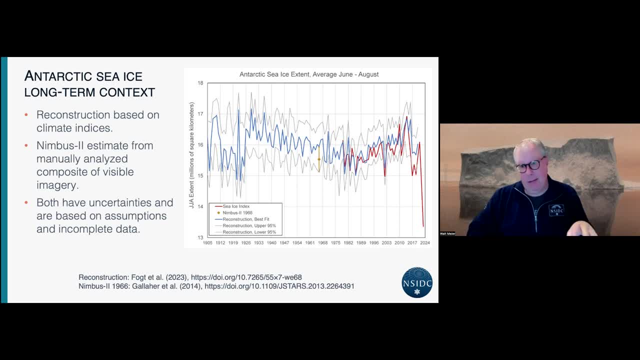 i said before, i think the august data is quite suspect and probably too low. but i did just, you know, for argument's sake, i took it as as we calculated, as it's published in the paper, averaged it with june and july, and that's what we get, and so that's within the 95 percentile of the reconstruction, and it's again. 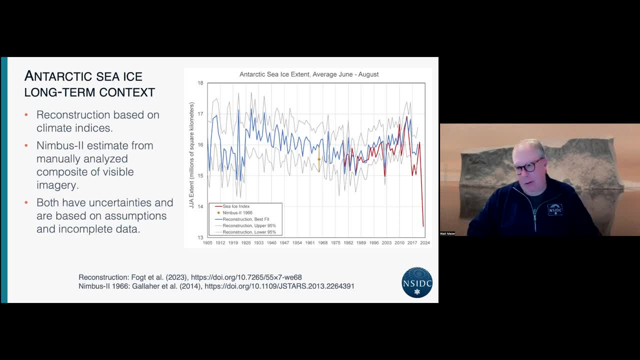 way above um. you know, a couple million square kilometers above um what we saw this year. so i, you know, this year it really is an outlier um based on anything that we can, we can put together. you know, reconstructions of course have uncertainties, and even that 95 percent bound. 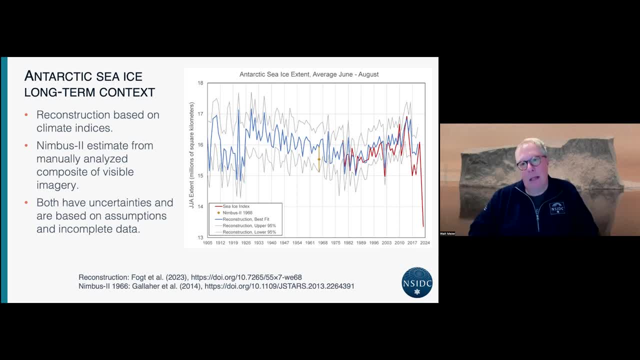 may not, you know, fully capture all the uncertainty that we have, and so i think that's what we're hoping to do, is to be able to understand the variability that may have happened in the antarctic. but i think, you know, looking at this, this is still very remarkable- uh, a year in terms. 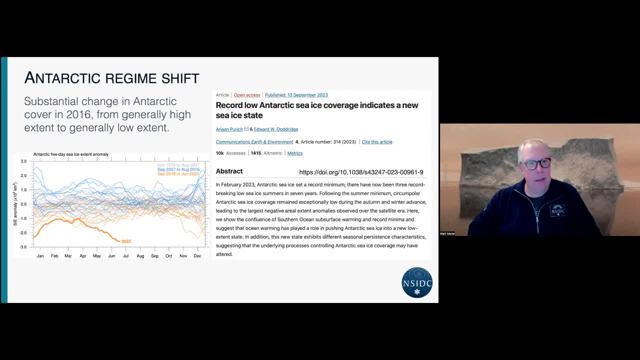 of, uh the antarctic, uh sea ice, um. so there's been a lot of talk about, um you know, the the sea ice coverage in the antarctic and what's going on and why it's happening. that's been a big question. um, we've actually seen- i think i mentioned before- a regime shift really starting uh. 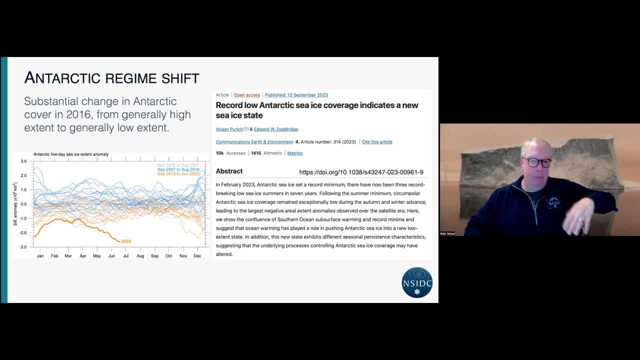 in like august to september of 2016, where it went from generally high, even record high levels within a couple years before, to low levels- um, generally low levels. and then this year is kind of the exclamation point on that, and there was a recent paper, uh by purich and doddridge- uh in nature. 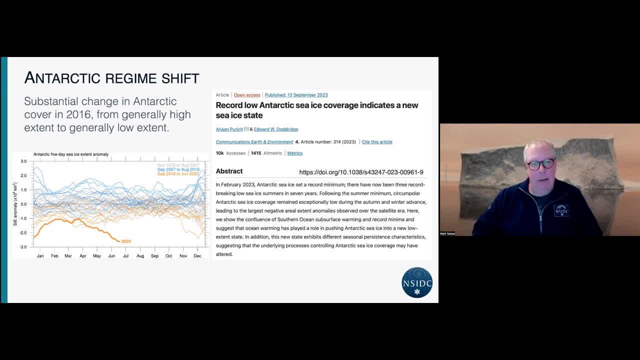 uh, communications, earth and environment. um, that, looked at this. they- they actually, you know, almost doing new real-time science here. they use the data through the epa and they used this information, uh, to kind of get more information about you know how things are more important in the current. yeah, i mean, that was a very interesting paper. 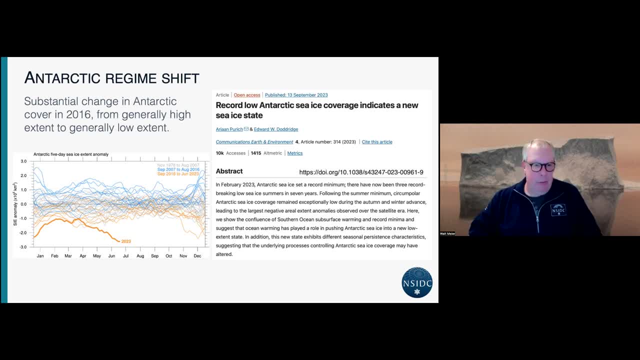 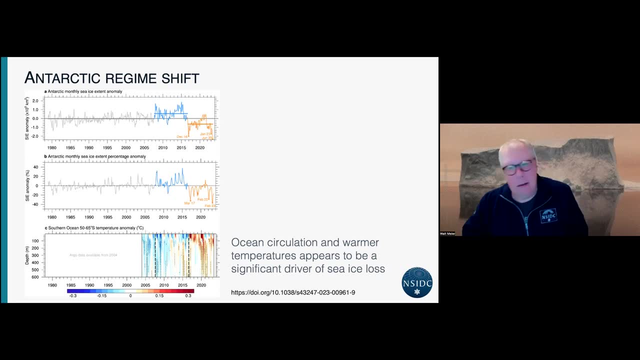 i think it was published in the state book. i think it was published in january, or maybe it was in january or in june 2023, um. but they also were looking, you know, kind of this 2016 forward regime shift, um, and what they see is is, uh, you know, again, this, this really general trend. towards less ice in that since 2016, and then this really extreme year in 2023, i think i've got, yeah, another um figure from that paper where again you see this: the top is the ca6 anomaly. it's generally high, at least from like. 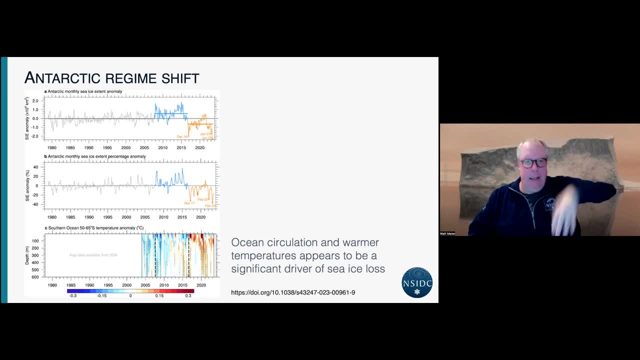 2007 through 2016, and then it drops low percent anomaly in the middle, and what they looked at was that ocean temperatures being much warmer in in the recent years, in these last seven years on average, and so you can see the not just the surface waters, but also even at depth, so it 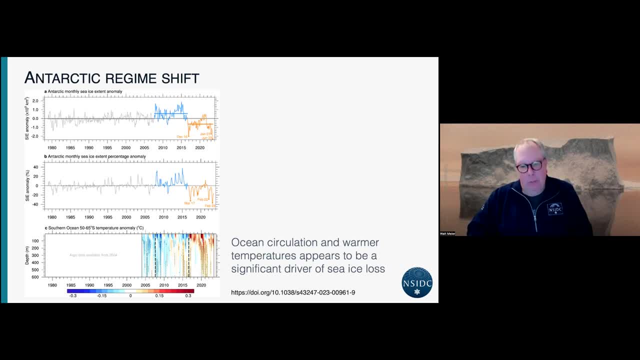 seems like ocean. uh, more warmer temperatures and warmer ocean temperatures and perhaps changes in circulation bringing that heat closer to the antarctic sea ice, basically prevented the ice cover from growing like it normally would. um this year, um, and really over the past seven years, um, i don't think they really have too much data from. you know that this summer, in terms of the ocean. 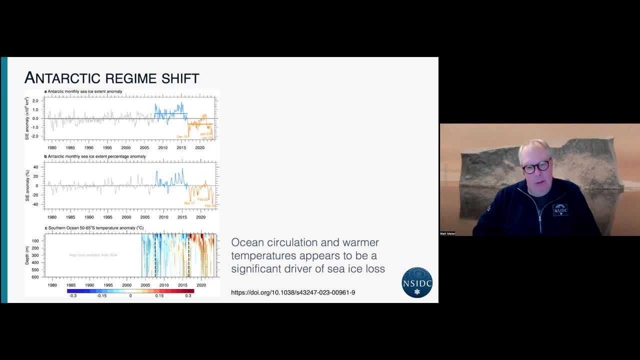 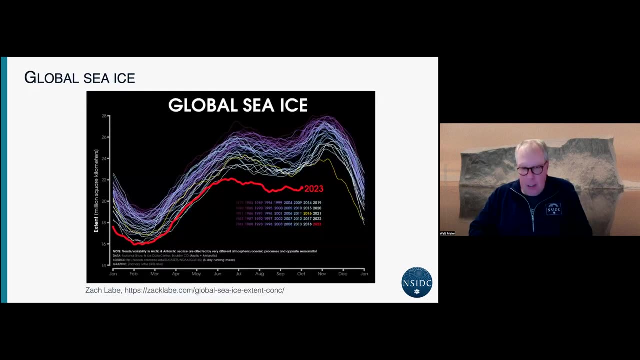 temperatures, but um, uh, but you know so it may even be more extreme than what's really shown here you for this summer, but it seems like the, the, the ocean temperatures and the ocean heat is a key player. there could be some atmospheric circulation patterns, um, but um, one of the 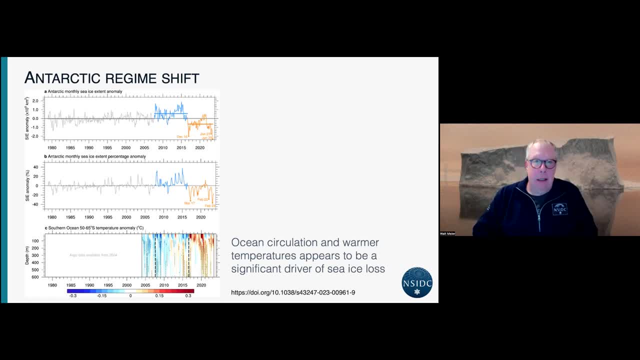 things that that's unique about this year is um the ice loss. we've seen years where there's been extremes in, like the weddell sea, or in the ross sea or the bellingshausen sea. we've seen a lot extreme bellingshausen sea, low ice years in the antarctic, over the. 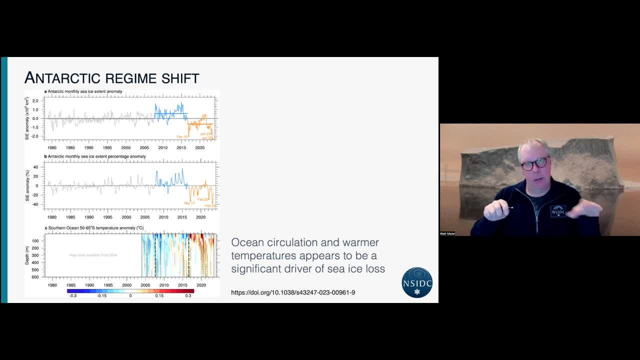 last 20 years or so um due to warm temperatures there and also circulation bringing in warm, warm air. but what typically we see in terms of atmospheric circulation is it will be really low in one area but higher in another area, so you get this kind of multimodal um. you know, high, low uh sea. 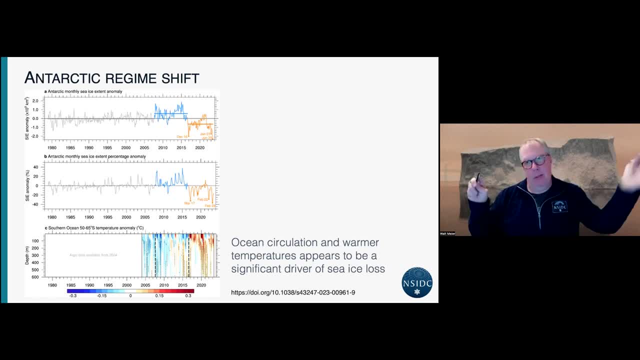 ice and that's not too surprising. you've got your circulation, that's. that's bringing warm air on one side. it's going to be cold air on the other side, and if it's pushing ice in from one side of a of a pressure system, it's going to be pushing it out on the other side, but the ocean heat can. 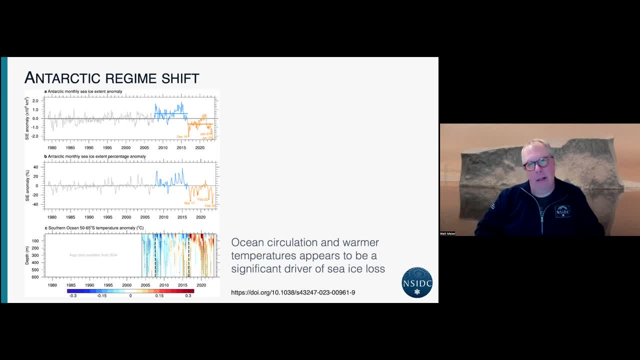 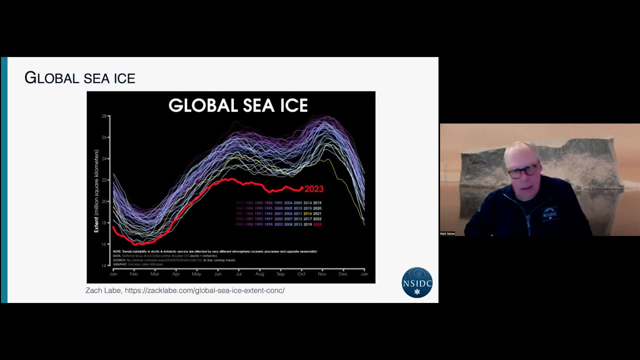 affect the entire uh circumference of the ice and that's what we saw this year. we're nearly everywhere in the antarctic, nearly every sector. it was below average um for throughout the winter growth season, um, and so that's. that's definitely a change from what we've seen, um kind of finish. 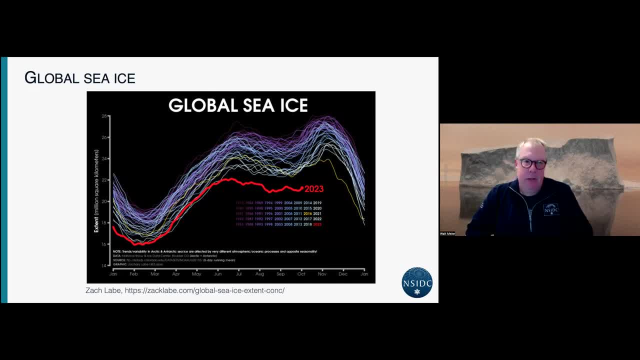 up quickly. uh, people have kind of pushed this global sea ice. i've been kind of reluctant to to talk about it but, um, i think with things being so extreme it's, it is kind of interesting to to look at. um, one of the things is that people would look at the global sea ice and use the 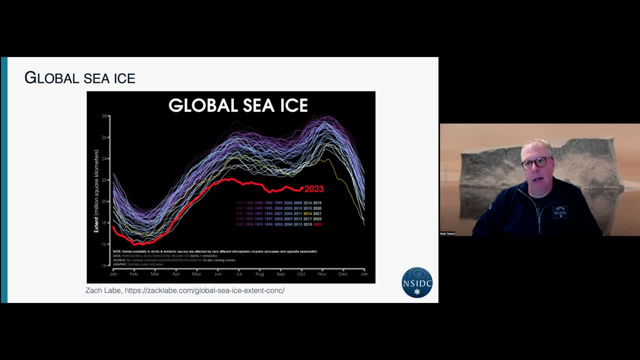 global sea ice as a as a retort towards the arctic sea ice. um, because we would have low arctic sea ice sometimes the antarctic would be higher and the global would be kind of more normal. so people would say, well, don't they cancel out. and that's of course not true. they're different. 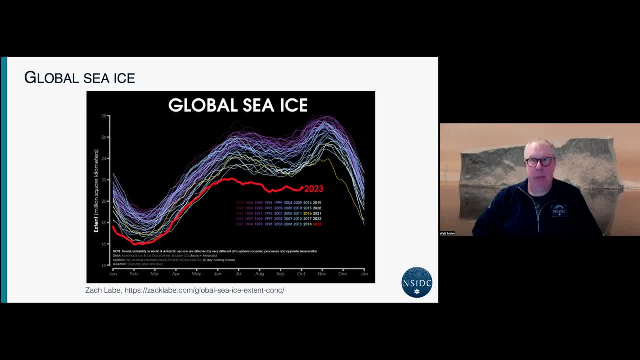 environments um, the antarctic kind of changes, the global sea ice- and that's of course not true because it's so much bigger, especially in the like september when it's at a maximum um, but now both are, you know um kind of low, and so it's really showing an extreme year. 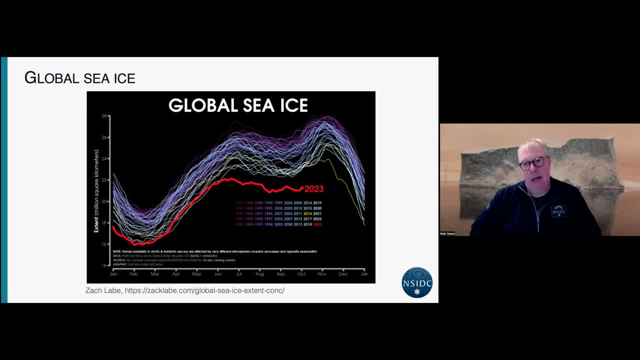 i don't want to like kind of cherry pick this just because it's in our favor now, so to speak, in terms of um now reinforcing that, the changes to both arctic and antarctic. um, i still think global sea ice is maybe not the best metric to use. it's better to look at each individual hemisphere. 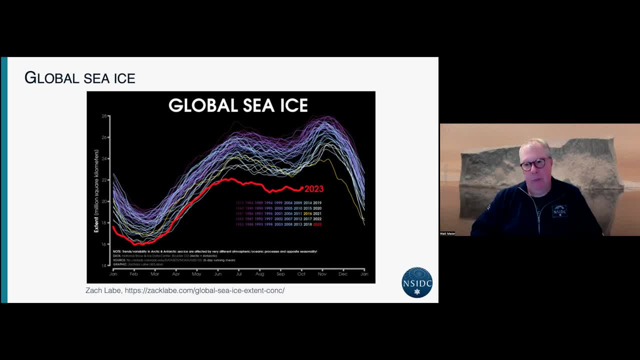 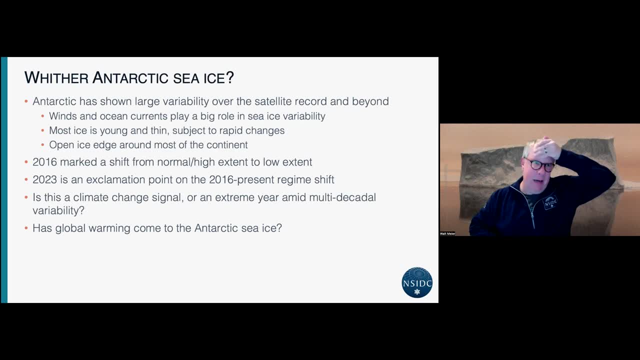 um, but it does kind of add yet another, you know, pretty stunning um point in terms of how things are are different than they used to be. so you know, the kind of the question that a lot of people are asking- and i'm sure people will be studying in the coming months, years- is you know what? what's? 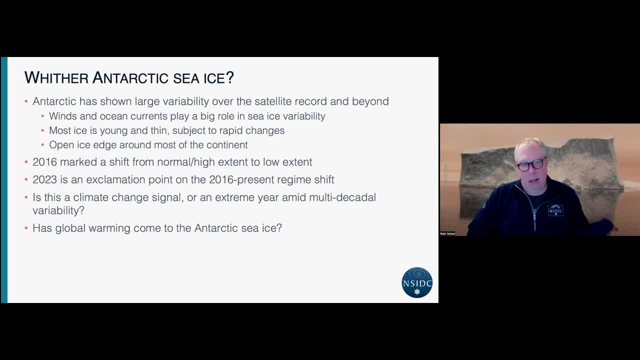 going to happen to antarctic sea ice? um, it's shown a lot of large variability over the satellite record and and beyond. winds and ocean currents play a huge role. um, you've got. the ice edge is completely open to the ocean nearly everywhere around the continent. um, it's got a. 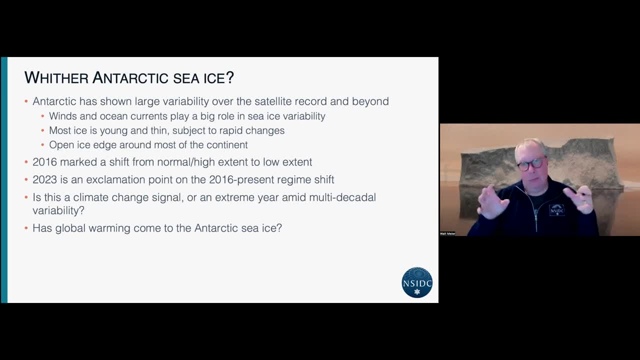 huge circumference, um at its maximum, so it's very sensitive to the whims of ocean currents and winds. the ice is young and thin as well, so again, it can change quite rapidly, um, and so you know this. there's there's a lot of room for things to vary um, but we have seen this, you know. now it's been. 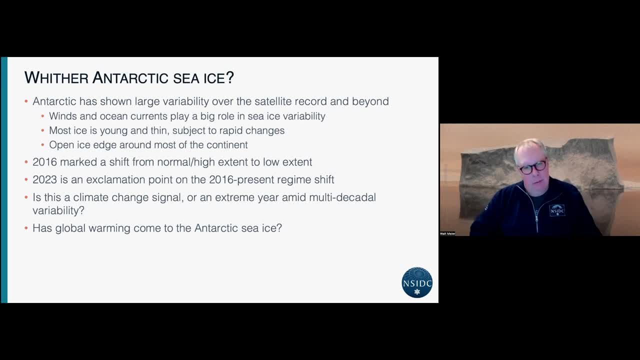 really been since 2016 that we've seen this regime shift towards generally lower expense. and then this year was, you know, just an exclamation point in that um, where it's just, you know, really low, and you know the question is is: is this just a really extreme year amid, you know, multi-decadal 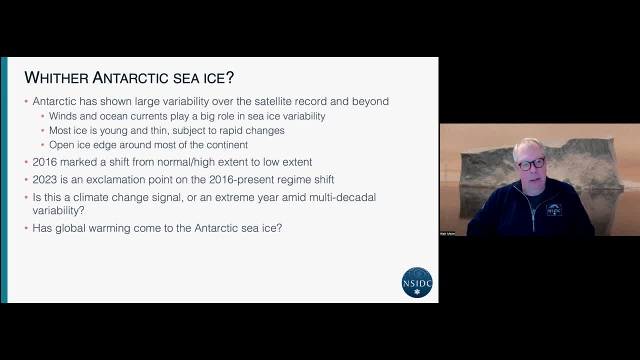 variability or is this really a climate change signal? um, you know, that is going to be something that's going to carry on in the future years and, you know, are we going to see the antarctic now starting to to behave and lose ice, like the arctic has been doing? um, in other words, you know.